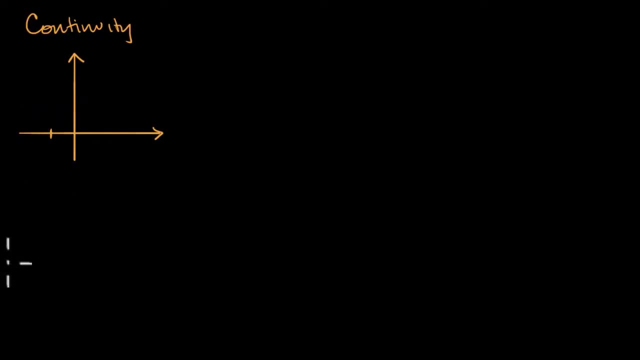 But if I had a function that looked somewhat different than that, if I had a function that looked like this: let's say that it is continuous and it is defined up until then, and then there's a bit of a jump, and then it goes like this: 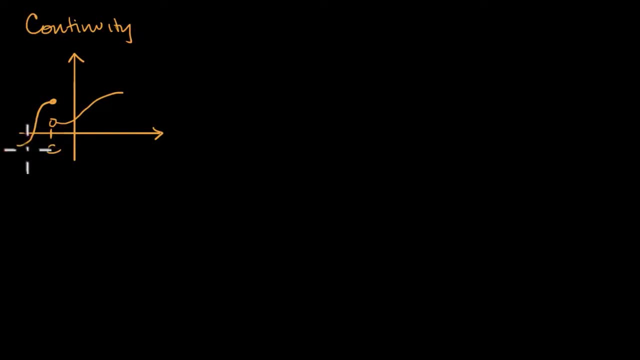 well, this would be very hard to draw. this function would be very hard to draw, going through x equals c, without picking up my pen. Let's see, my pen is touching the screen, touching the screen, touching the screen. How do I keep drawing this function without picking up my pen? 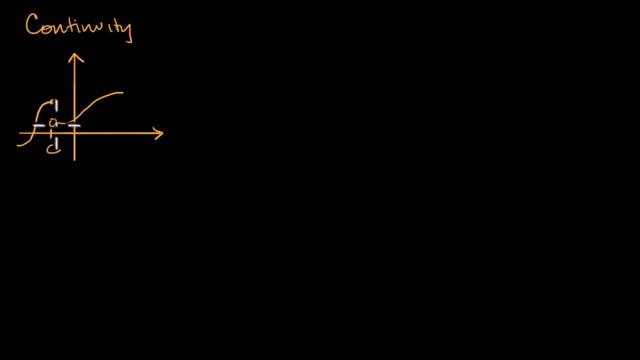 I would have to pick it up and then move back down here, And so that is an intuitive sense that we are not. we are not continuous in this case, right over here, But let's actually come up with a formal definition for continuity. 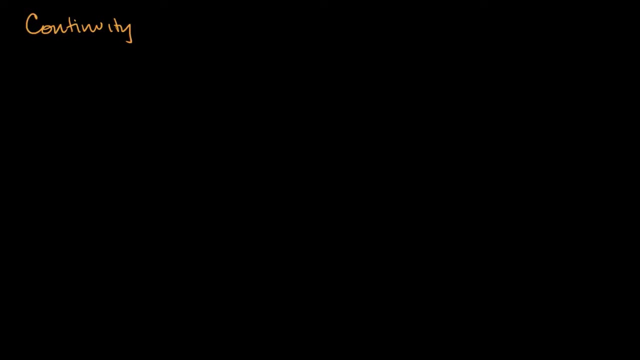 and then see if it feels intuitive for us. So the formal definition of continuity. let's start here. we'll start with continuity at a point. So we could say: the function f is continuous. continuous at x equals c if, and only if. 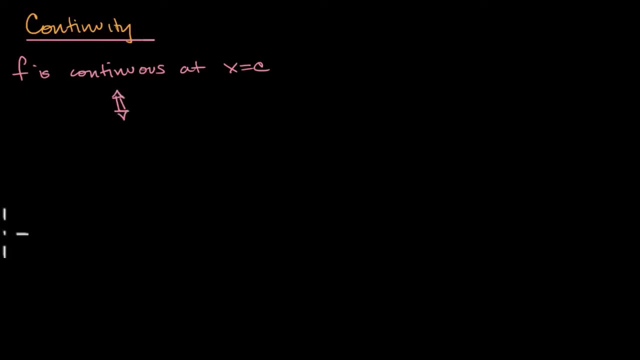 I'll draw this two-way arrow to show if, and only if, the two-sided limit of f of x as x approaches c is equal to f of c. So this seems very technical, but let's just think about what it's saying. It's saying: look, if the limit as we approach c from the left and the right of f of x, 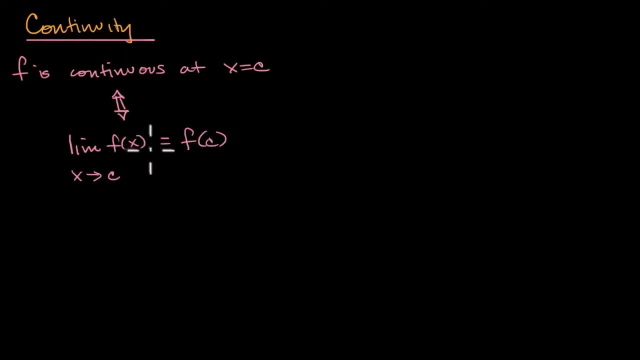 if that's actually the value of our function there, then we are continuous at that point. So let's look at three examples. Let's look at one example where, by our picking up the pencil idea, it feels like we are continuous at a point. 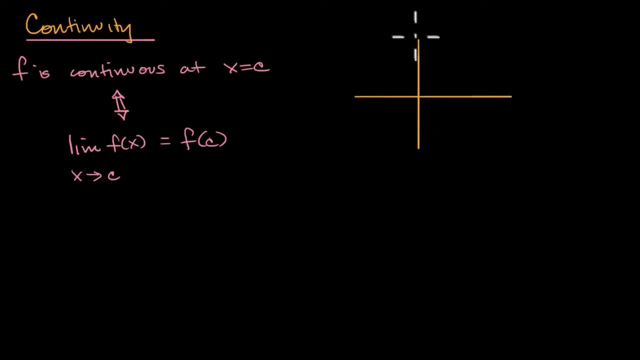 And then let's think about a couple of examples where it doesn't seem like we're continuous at a point and see how this more rigorous definition applies. So let's say that my function- so let's say this right over here- is: y is equal to f of x. 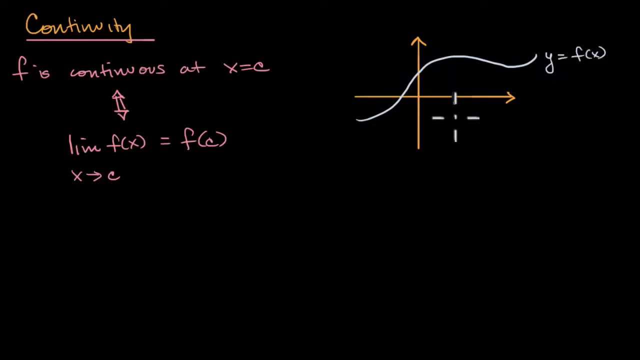 and we care about the behavior right over here when x is equal to c. This is my x-axis, That's my y-axis. So we care about the behavior when x is equal to c. And so notice from our first intuitive sense. 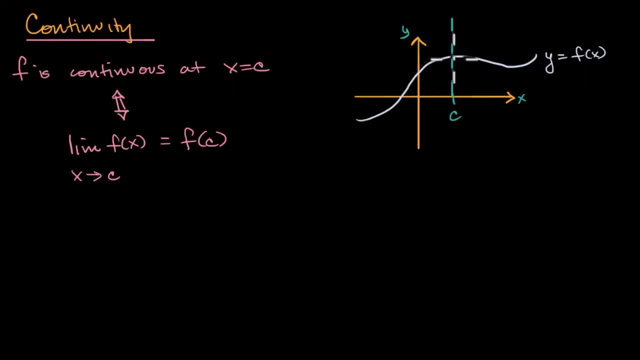 I can definitely draw this function as we go through x equals c without picking up my pencil. So it feels continuous there. There's no jumps or discontinuities that we can tell. It just kind of keeps on going. It seems all connected is one way to think about it. 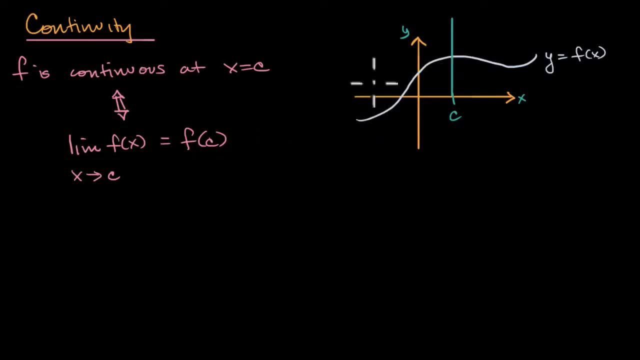 But let's think about this, Let's think about this definition. Well, the limit as x approaches c from the left, it is: as we approach from the left. it looks like it is approaching. it looks like it is approaching f of c. 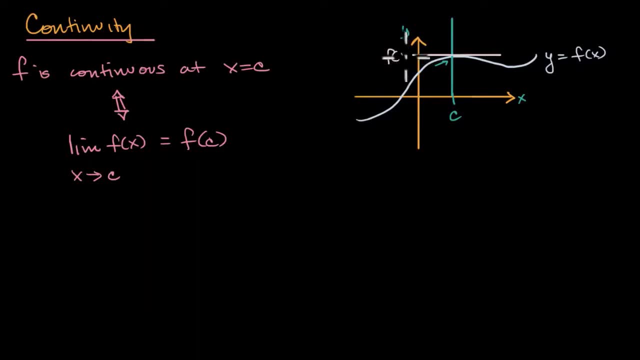 So this is the value f of c, right over here And as we approach from the right, as we approach from the right, it also looks like it's approaching f of c And we are defined right at x equals c And it is the value that we are approaching. 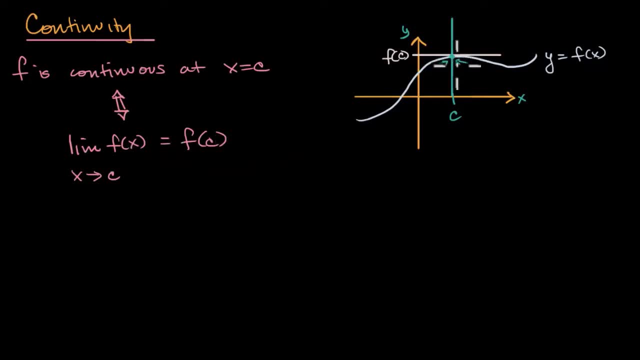 from both the left or the right. So this seems good in this scenario. So now let's look at some scenarios that we would have to pick up the pencil as we draw the function through that point, through that, through that, when that. 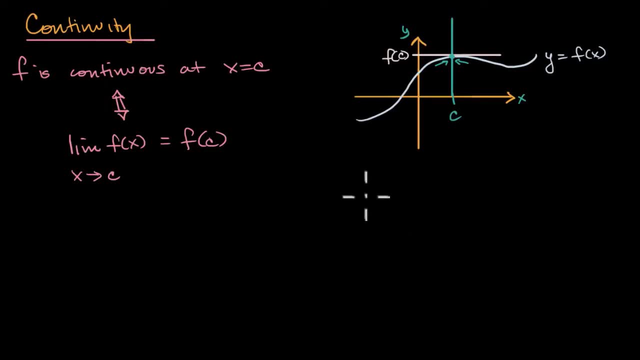 when x is equal to c. So let's look at a scenario. Let's look at a scenario where we have what's often called a point discontinuity, so we don't have to know at this point- not no pun intended- the formal terminology for it. 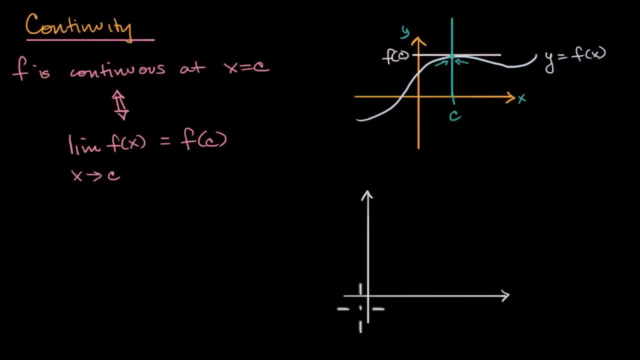 So let's say we have a function that, let's see, this is c, And let's say our function looks something, something like this, So we go like this, And at c let's say it's equal to that. So f of c is right over here. 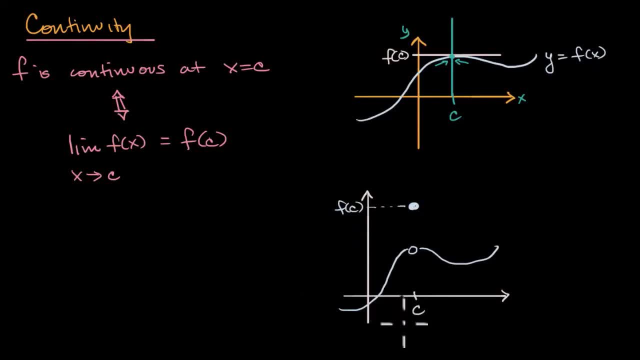 f of c would be that value. But what's the limit as x approaches c? So the limit as x approaches c, and this would be a two-sided limit of f of x. Well, this is as we approach from the left. it looks like we are approaching. 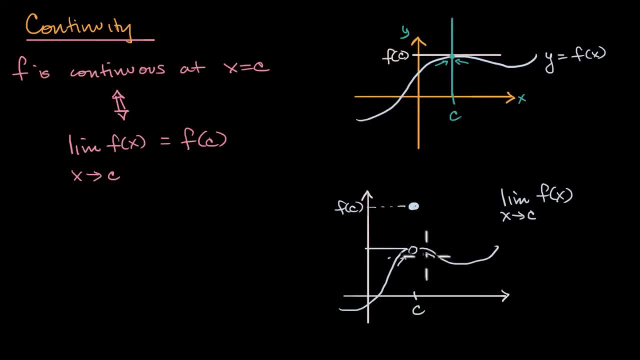 this value. right over here, And from the right, it looks like we are approaching that same value, And so we could call that l, And l is different than f of c, And so in this case, by our formal definition, we will not be continuous at. 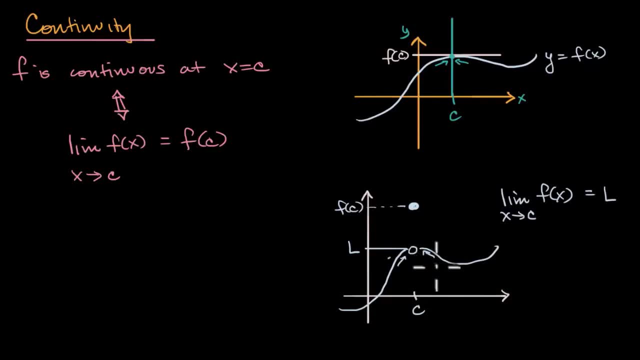 f will not be continuous. for x, We will be at the point x or when x is equal to c, And you could see that there, If we tried to draw this. okay, my pencil is touching the paper, touching the paper, touching the paper. 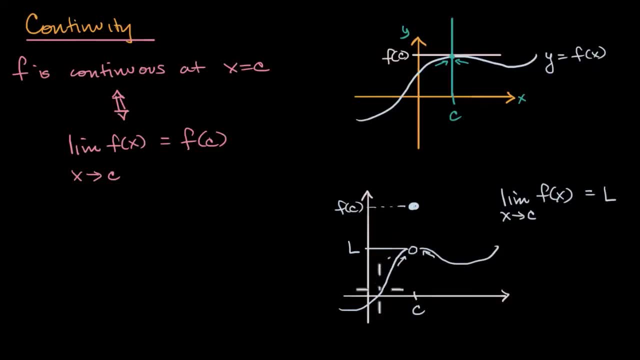 Uh-oh, if I needed to keep drawing this function, I'd have to pick up my pencil, move it over here, then pick it up again and then jump right back down. But this rigorous definition is giving us the same conclusion. 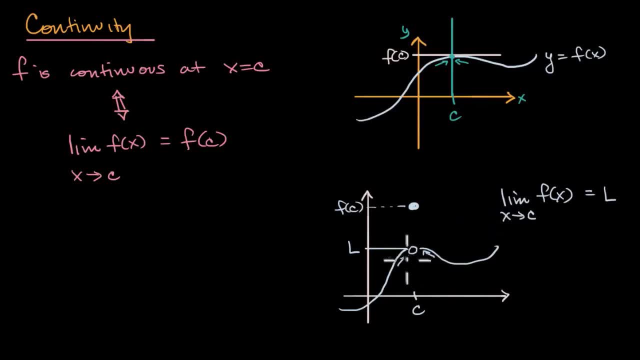 The limit as we approach. x equals c from the left and the right. it's a different value than f of c, And so this is not continuous, Not not continuous. And let's think about another scenario. Let's think about a scenario. 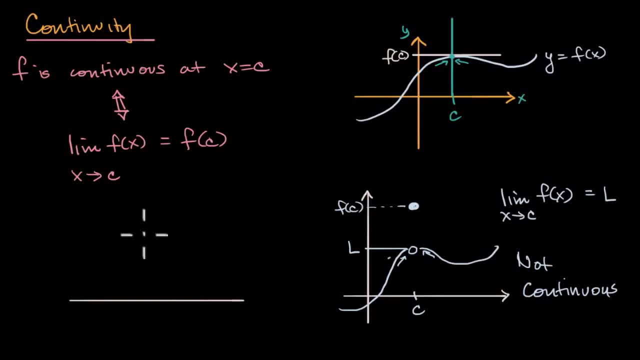 and actually maybe let's think about a scenario where the limit, the two-sided limit, doesn't even exist. So there are my axes x and y And let's say it's doing something like this. Let's say it's doing something like this: 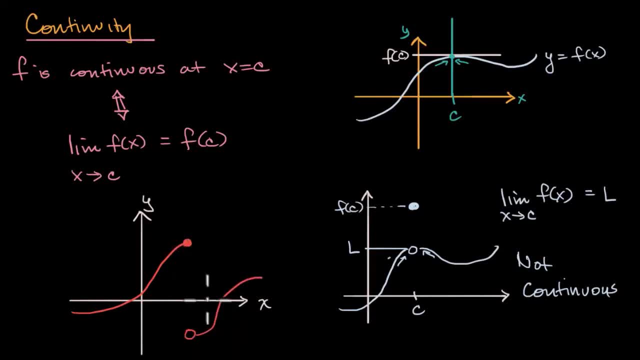 And then it does something like this and goes like that And let's say that this right over here is our c, And so let's see, this is f of c right over here. That is, let me draw it a little bit neater. 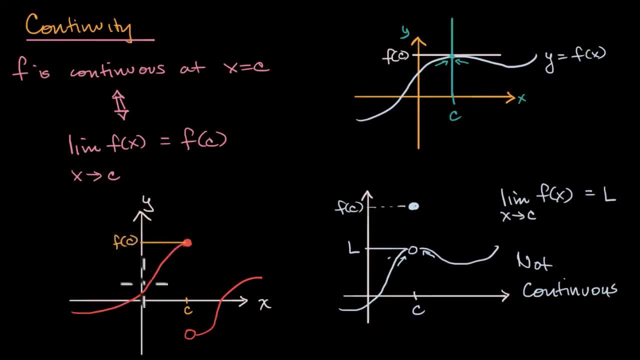 That is f of c And it does look like the limit as x approaches c from the left. so from values less than c, it does look like that is approaching f of c, But if we look at the limit as x approaches c from the right, 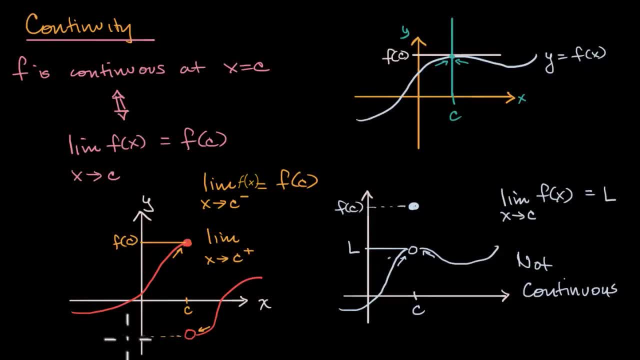 that looks like it's approaching some other value. That looks like it's approaching this value right over here. Let's call it l. That's approaching l, and l does not equal f of c, And so in this situation, the two-sided limit doesn't even exist.